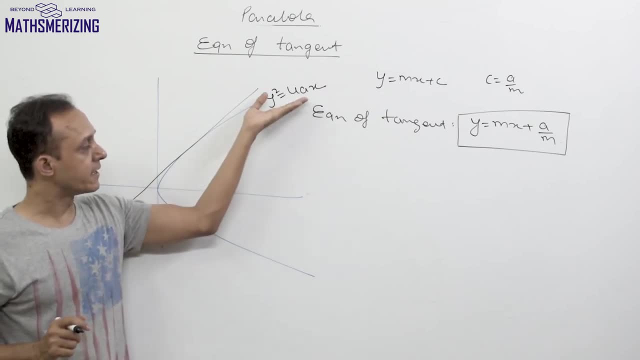 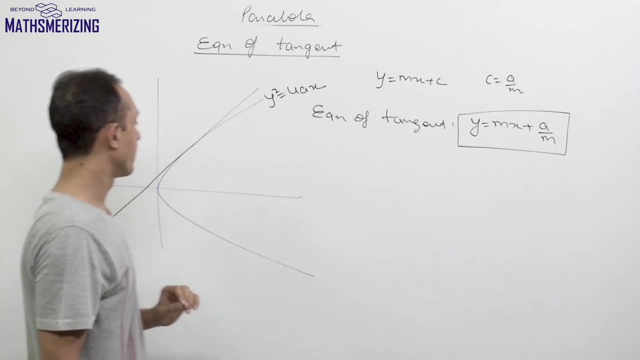 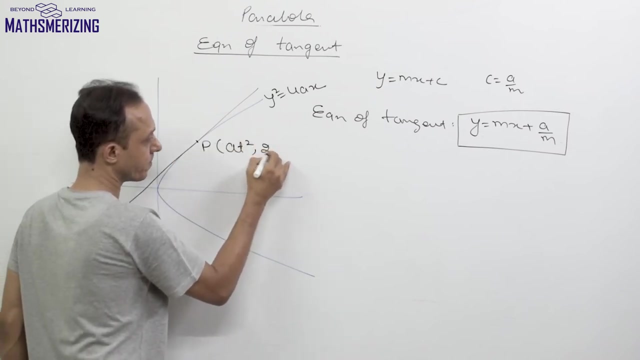 So if we have slope and if we have this equation, then we can simply write equation of tangent to this parabola as y equals mx plus a by m. Now another way of writing this equation of tangent is in terms of its parametric coordinate. So suppose, if I will say, point of contact of this tangent is suppose p and this is at square and twice at. 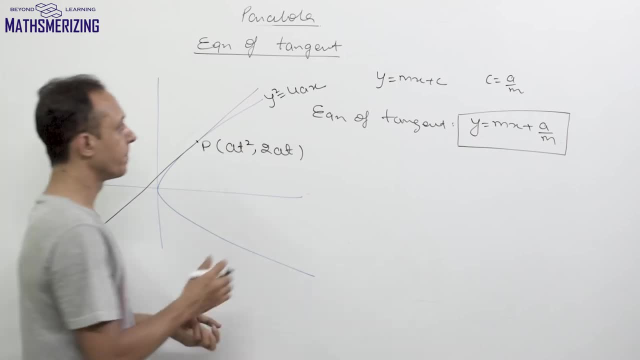 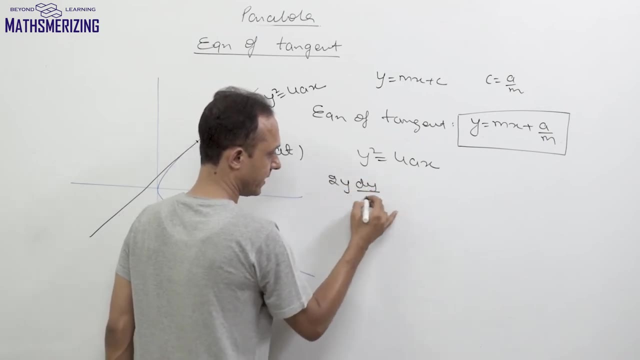 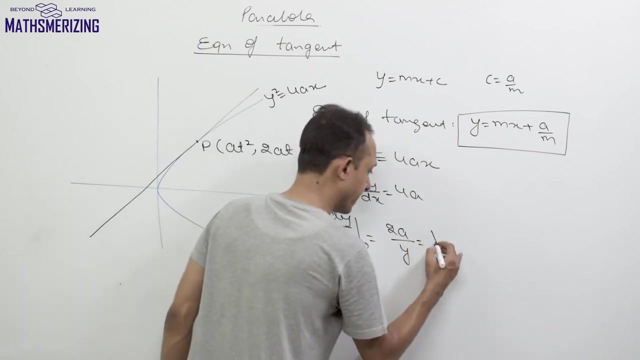 Now we can use calculus to find slope of this tangent. We know that for this parabola y square equals 4ax, So we will differentiate. we will get 2y. dy by dx is equal to 4a, So we will find dy by dx at this point p. So dy by dx at this point p will be 2a upon y. and what is the value of y? y in this case is twice at, So it will simply be 1 upon t. 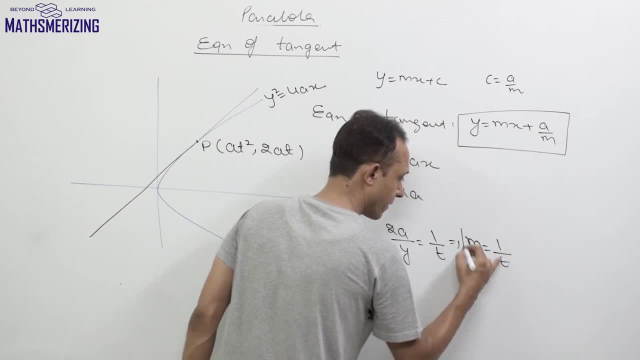 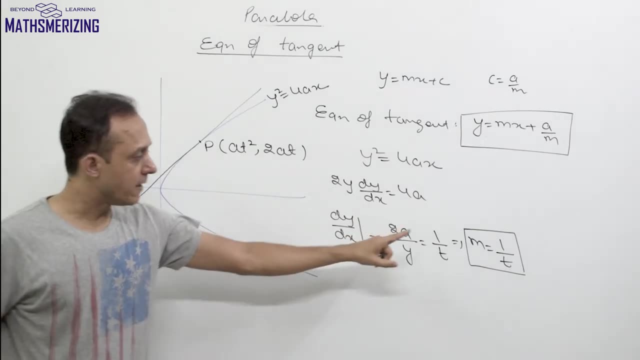 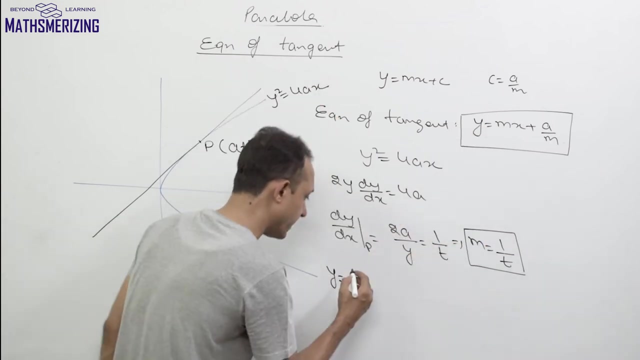 So that means slope of tangent. at any point, point a t square twice a, t will simply be 1.. So if we replace m with 1 upon t, we can write equation of tangent as y equals and in place of m I write 1 upon t, so it will be 1 upon t x. 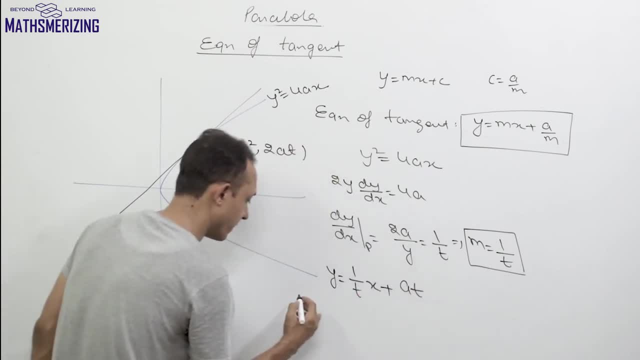 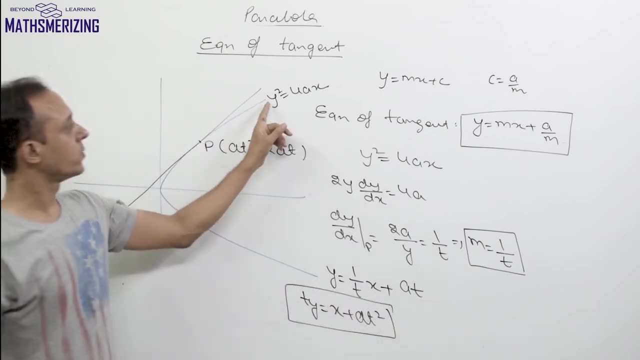 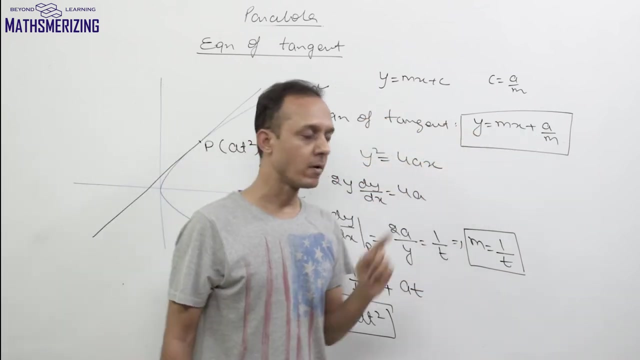 and then plus a t. So we can simply write it as ty equals x plus a t square. So for this parabola y square equals to 4ax. we can write equation of tangent as either in terms of slope, which is y equals m, x plus a by m, or in terms of its parameter, t, which is ty equals x plus a t square. 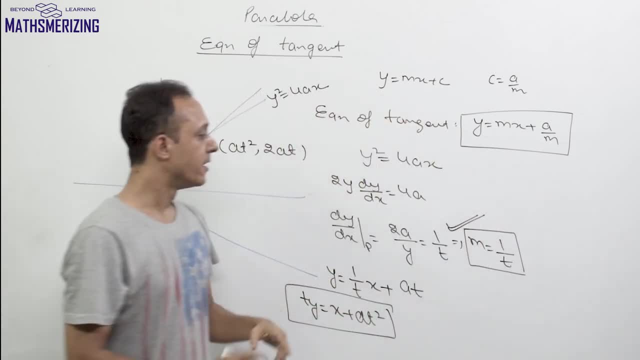 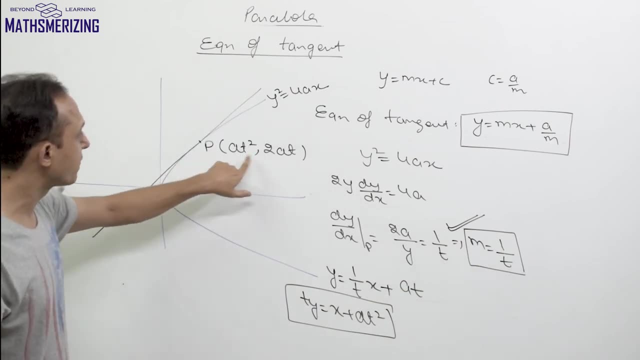 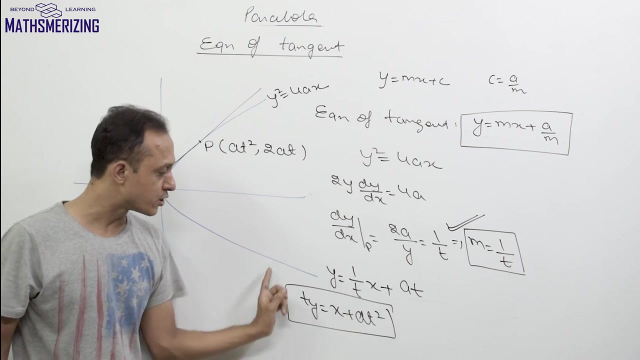 and we know that relationship between m and t is slope of this tangent should be 1 upon t. So for a parabola, if I know this parameter t, we can write this point of contact also, and then we can write equation of tangent also which is: ty equals x plus a t square. So when we'll be proving questions on 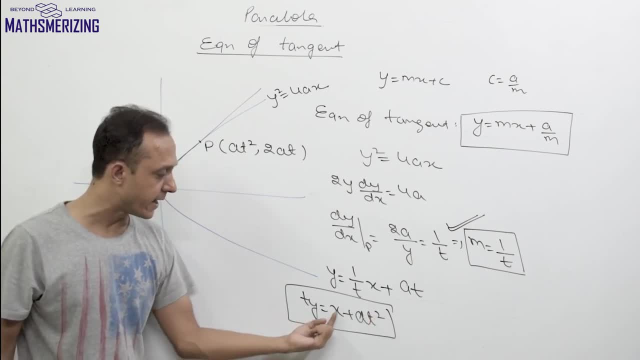 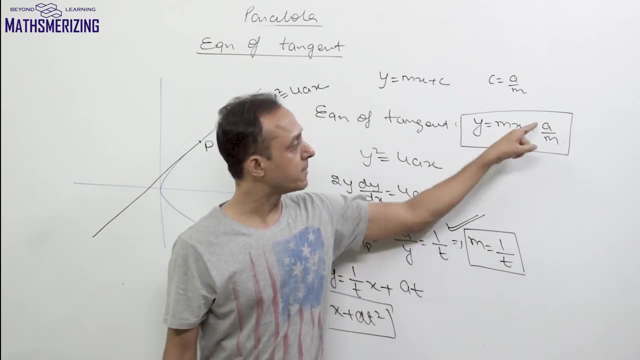 parabola, we'll be mostly taking this equation, which is ty equals x plus a t square. But when we are given slope of a tangent, then in that case we'll use this equation, which is y equals m, x plus a by m, where m is slope of this tangent. If I'm given slope of this tangent, I can.